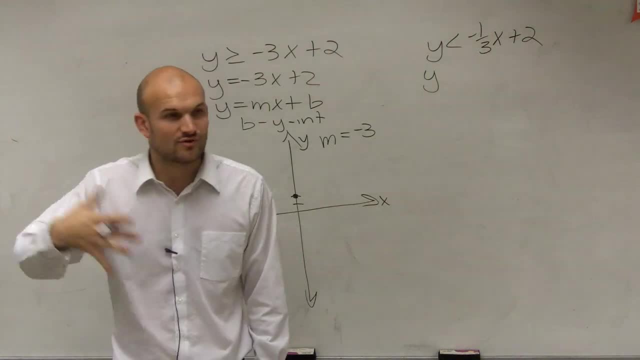 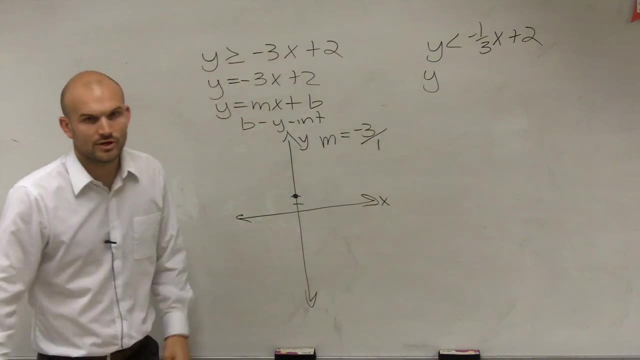 the number, But remember, slope right. a lot of times we say rise over run, change in y over change in x, So we want to write it as a fraction. Well, if it's not a fraction, just put it over 1, because 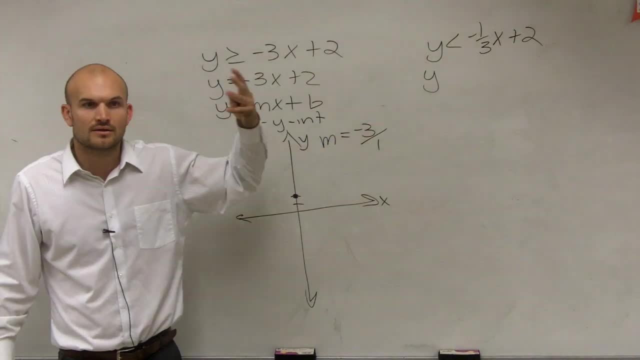 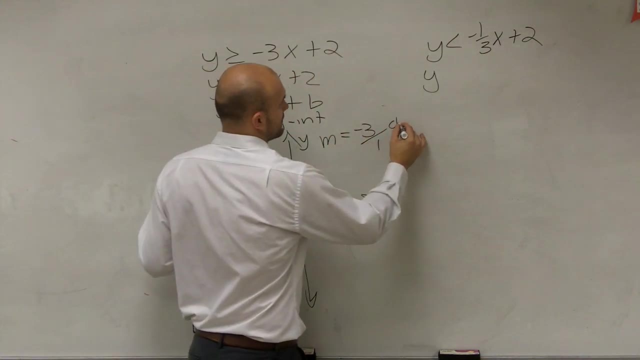 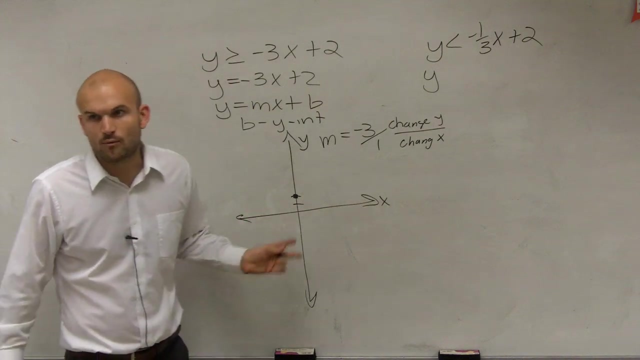 what's 1 divided by what's 1 divided into negative 3? Negative 3.. So now, what does negative 3 tell us? Remember it's the change in y over the change in x. So you can say: if my change in my y coordinates, 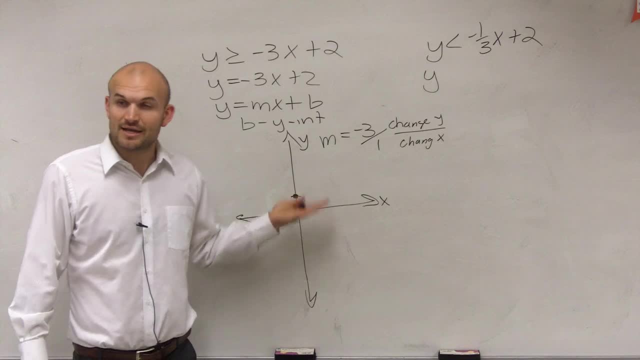 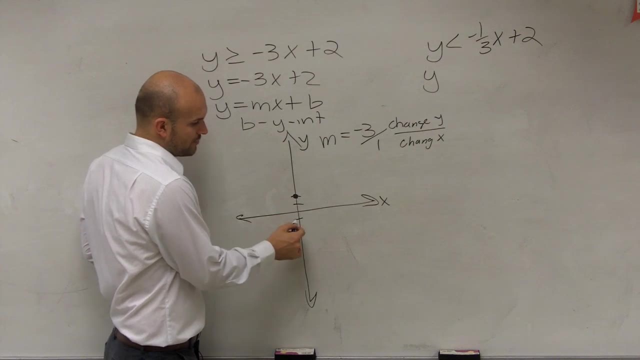 between one point and another. if that change is negative. 3, am I going to go up 3 or down 3? Down 3.. So you can go down 3.. So from this point, I go down 3.. 1,, 2,, 3.. 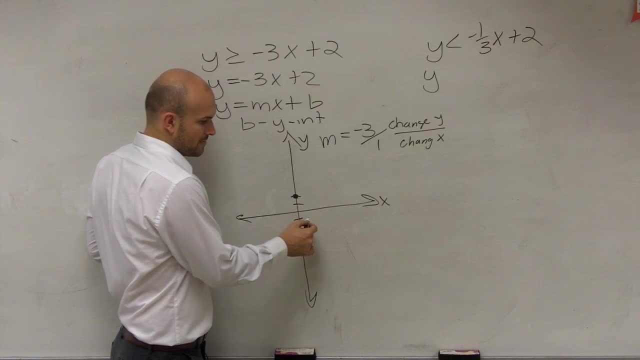 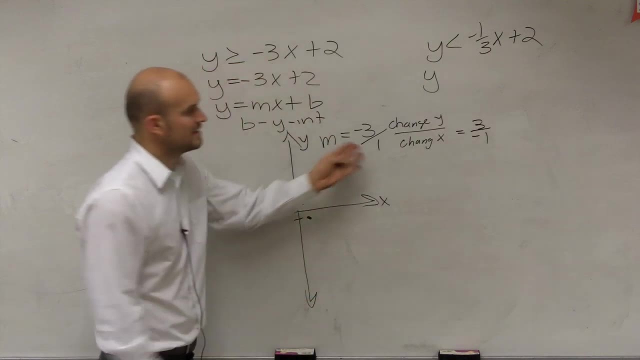 Then my change in x is positive 1.. So I'm going to go to the right one. Now just be careful: You could also write this as 3 over negative 1.. Negative 3 divided by 1 is negative 3.. 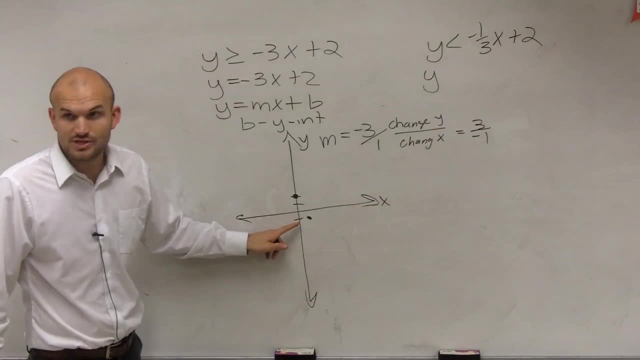 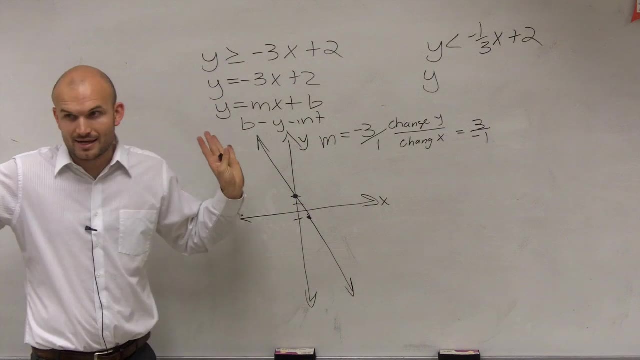 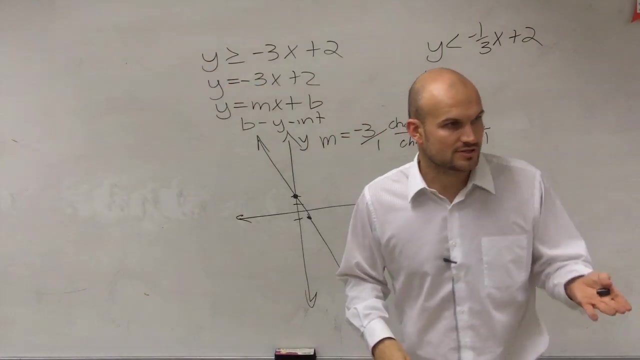 3 divided by negative 1 is also negative 3.. So you guys look at it. I connect my points. There's my line Done. Now we haven't done the inequality symbol Graph, the line first. Trevor, you got that. 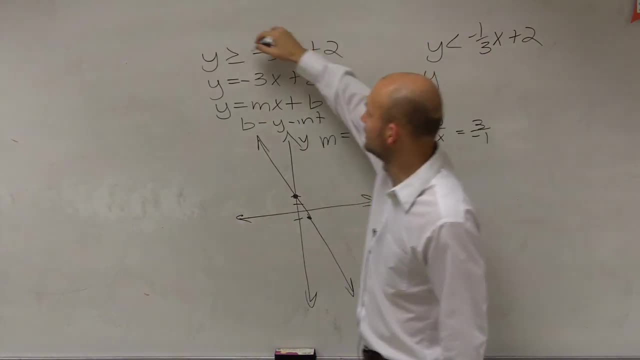 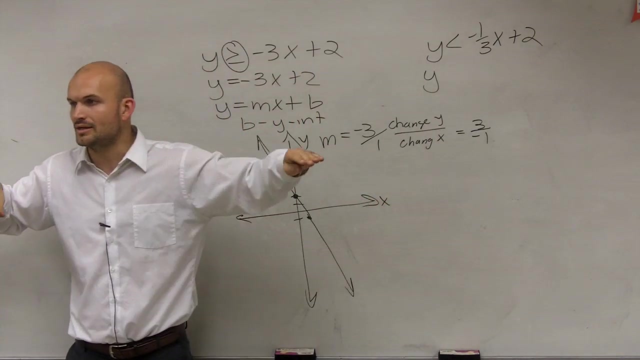 Graph the line. Now, what we need to do is we need to go back and look at our inequality symbol. Remember, guys, when we were graphing just one step or one variable inequalities? remember when we had the greater than or equal to, or less than or equal to? 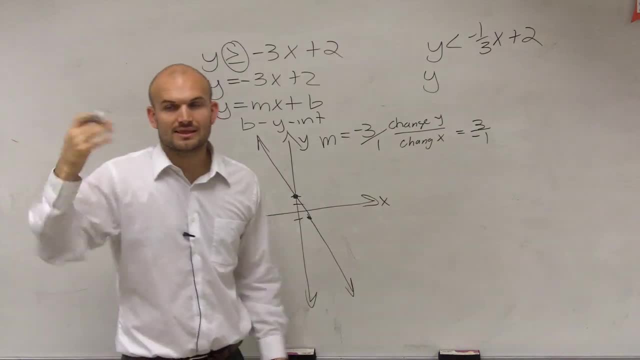 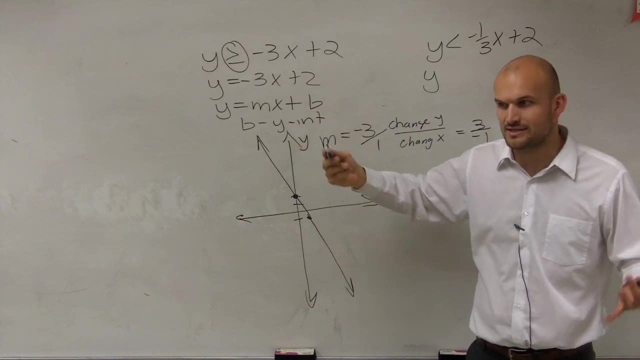 was that a solid dot or an open dot? Solid, Solid. So in lines we either do a dashed or a solid line. So should this be a solid line or a dashed, Solid, right, Just like it would be a solid dot. 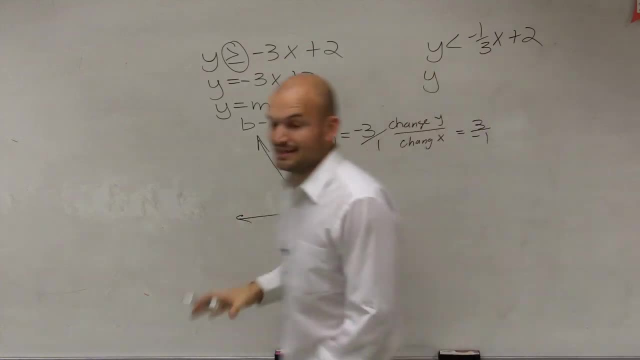 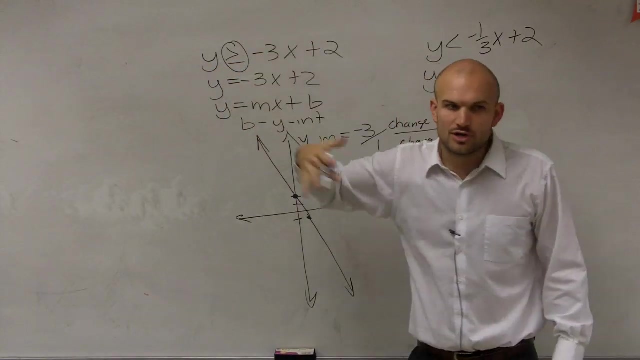 Yes, Hold on, Let me finish this video. Then the next thing we would talk about is test points. Remember shading. We always pick the point. Whenever you guys see inequality, you should always need to know we have to have shading. 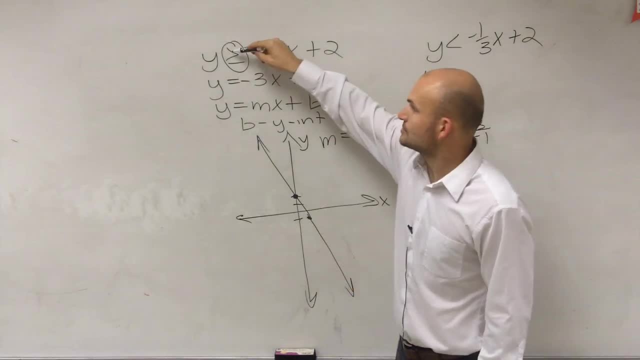 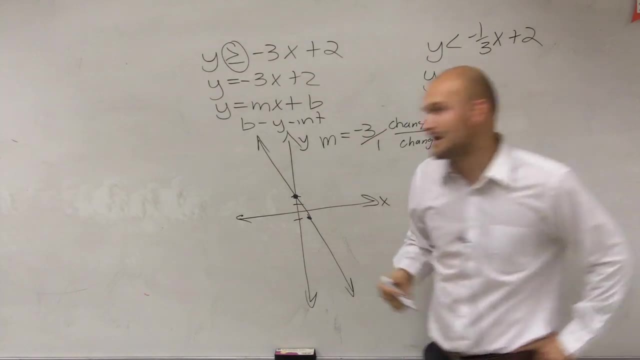 If I don't have shading, my problem's wrong. All right, So I have. n is greater than So we need to pick a test point. Does anybody remember the best test point ever I pick in the creation of man? Zero comma zero. 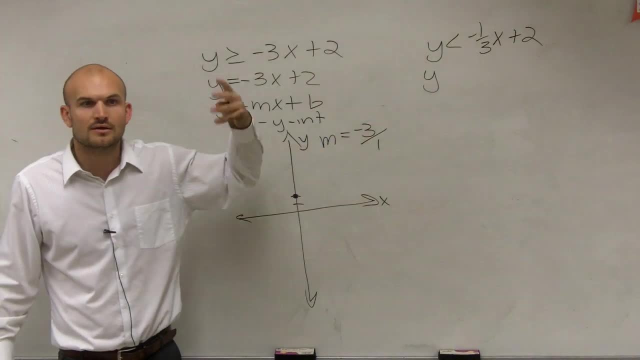 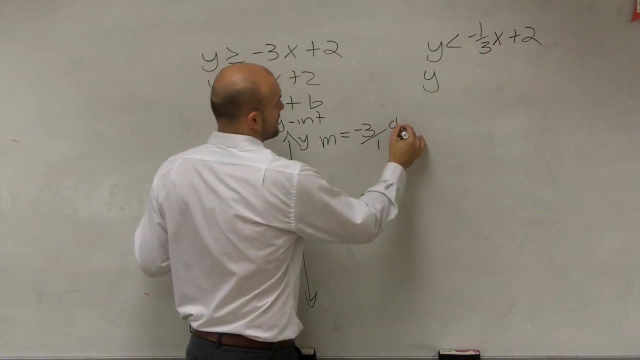 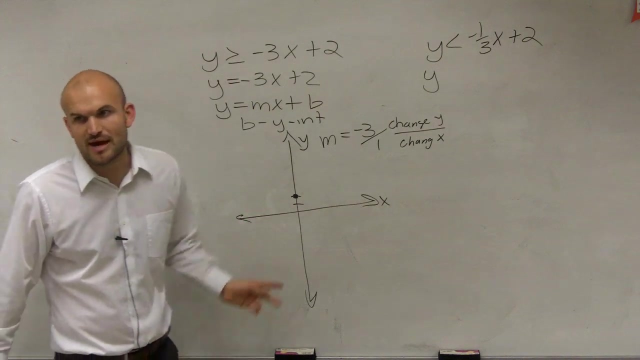 because what's 1 divided into negative 3? Negative 3.. Negative 3.. So now, what does negative 3 tell us? Remember it's the change in y. Does it change in x Over the change in x? So you can say if my change in my y coordinate is between one. 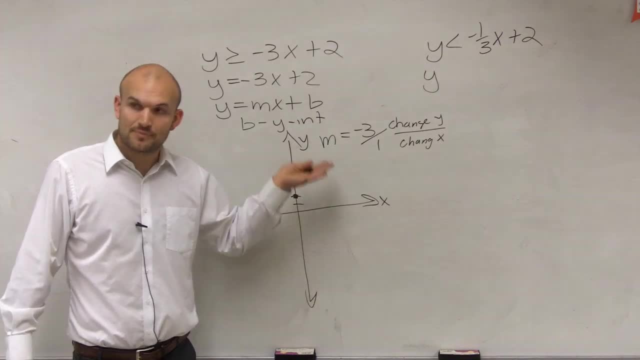 point and another: if that change is negative, 3, am I going to go up 3 or down 3? Down 3.. So you can go down 3.. So from this point, I go down 3.. 1,, 2,, 3.. 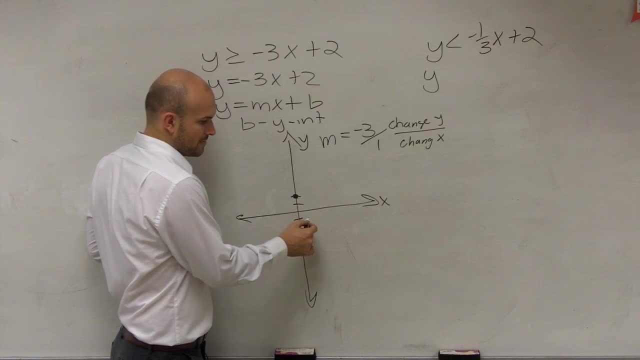 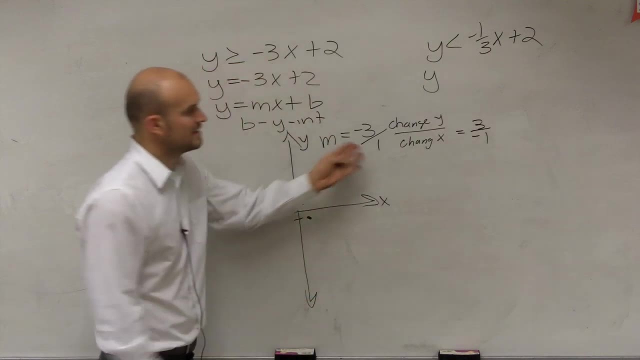 Then my change in x is positive 1.. So I'm going to go to the right one. Now just be careful: You could also write this as 3 over negative 1.. Negative 3 divided by 1 is negative 3.. 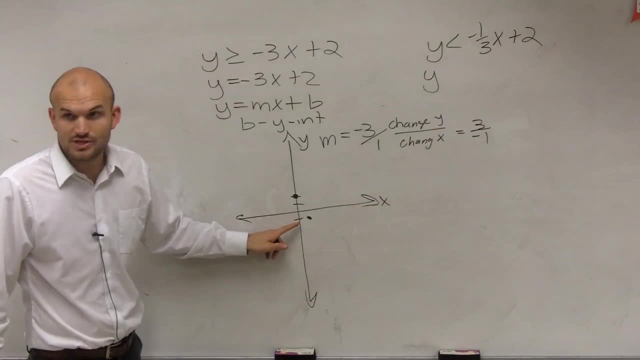 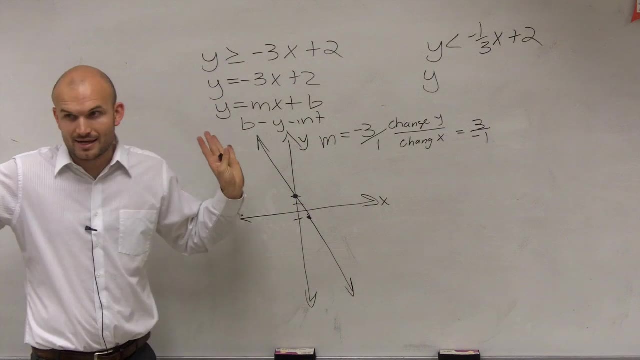 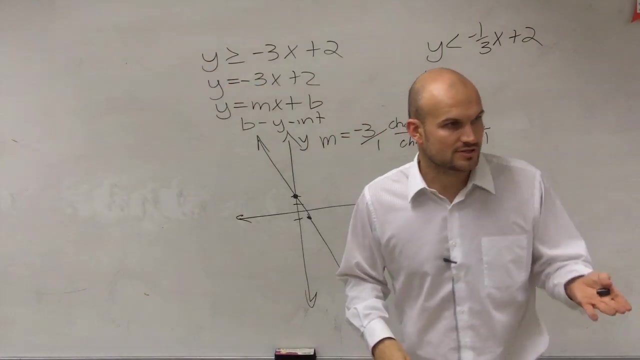 3 divided by negative 1 is also negative 3.. So you guys look at it. I connect my points. There's my line Done. Now we haven't done the inequality symbol Graph, the line first. Trevor, you got that. 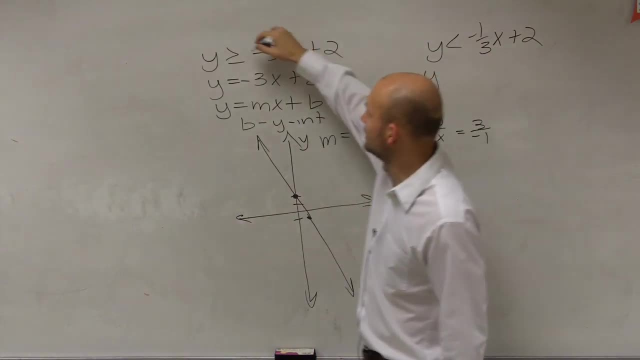 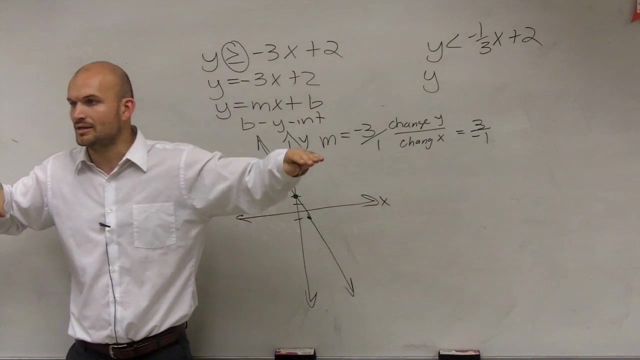 Graph the line. Now, what we need to do is we need to go back and look at our inequality symbol. Remember, guys, when we were graphing just one step or one variable inequalities? remember when we had the greater than or equal to, or less than or equal to? 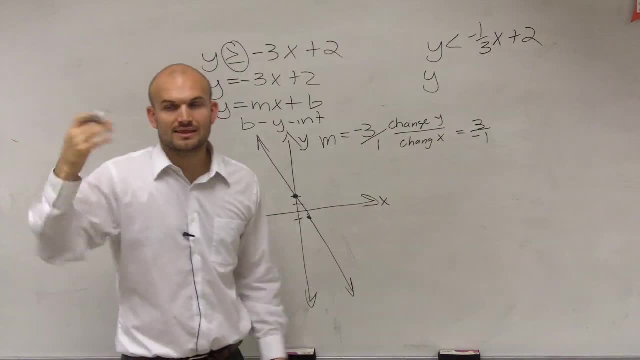 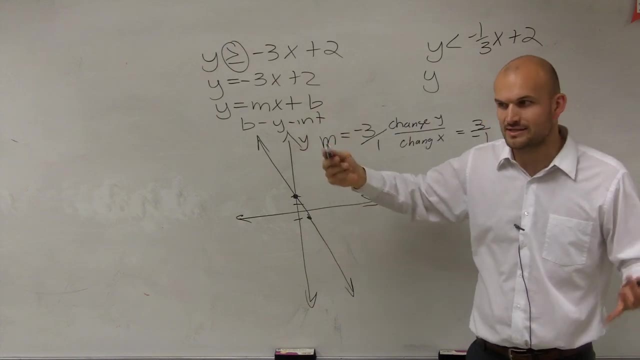 was that a solid dot or an open dot? Solid, dot, Solid. So in lines we either do a dashed or a solid line. So should this be a solid line or a dashed, Solid, Solid, right, Just like it would be a solid dot. 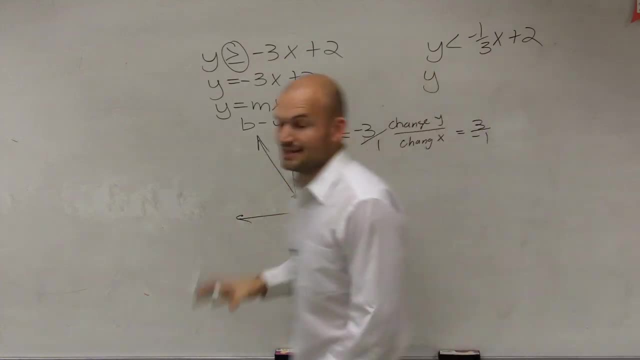 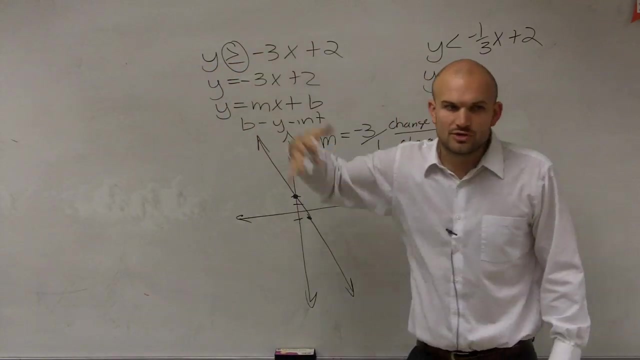 Yes, Hold on, Let me finish this video. Then the next thing we would talk about is test points. Remember shading. We always pick the point. Whenever you guys see inequality, you should always need to know we have to have shading. 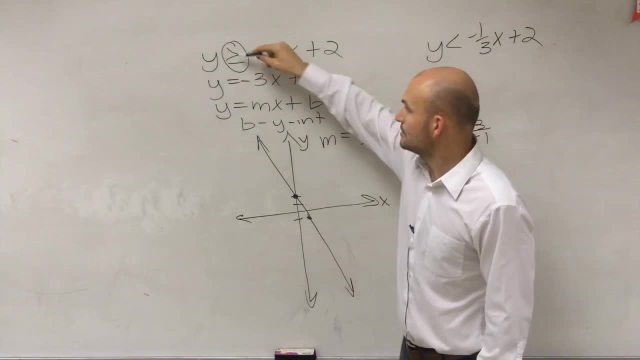 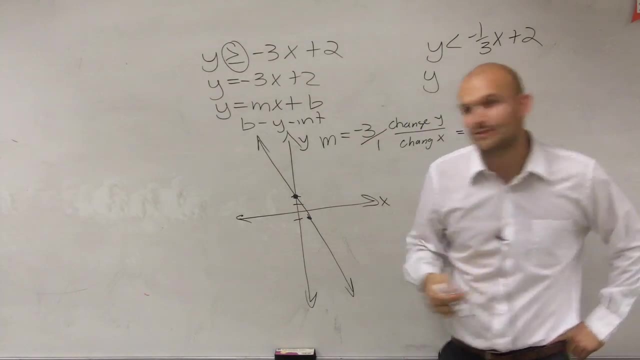 If I don't have shading, my problem is wrong. All right, So I have. n is greater than So we need to pick a test point. Does anybody remember the best test point ever? I pick in the creation of man: Zero comma zero. 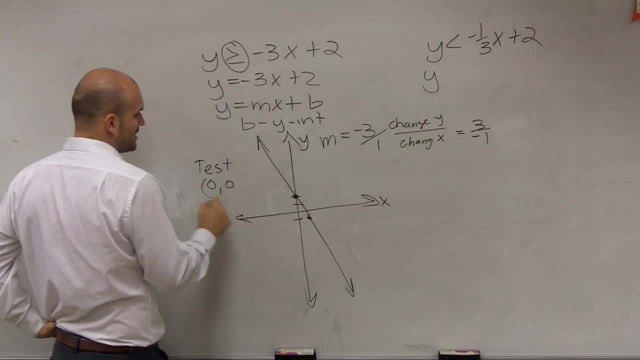 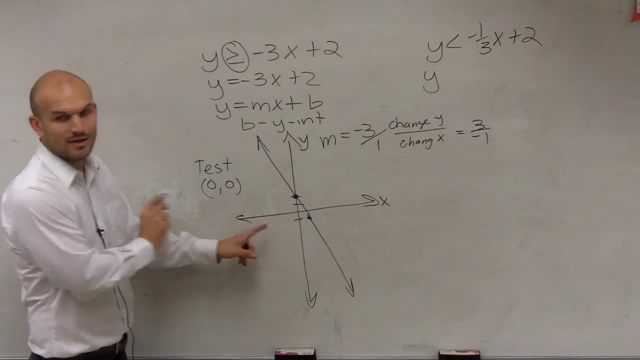 But the only time not to pick zero comma zero is when your line goes through zero comma zero. Does my line go through zero zero? No, No. So then, Mallory, all I do- What do you pick for- goes through zero zero. 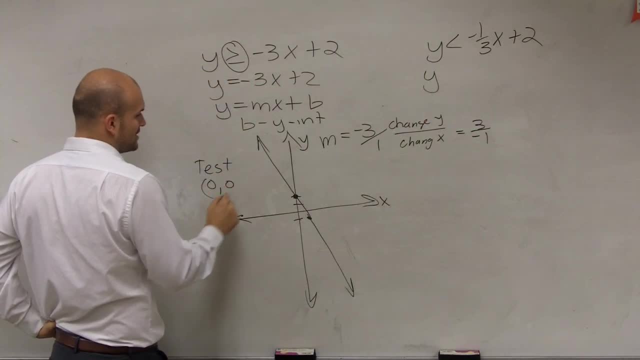 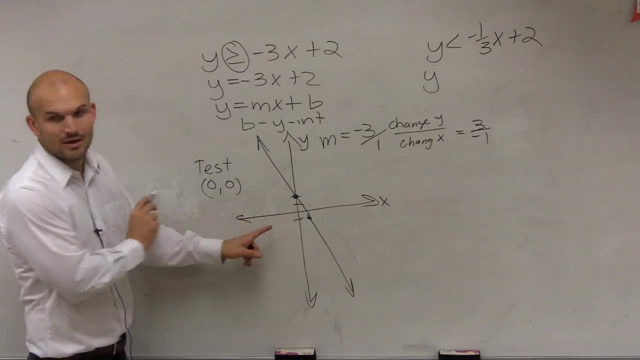 But the only time not to pick zero comma zero is when your line goes through zero comma zero. Does my line go through zero zero? No, No. So then, Mallory, all I do- What do you pick for- goes through zero zero.